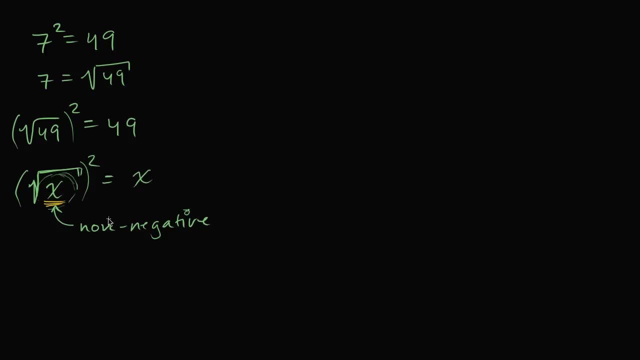 because it's hard to square a number, at least the numbers that we know about. it's hard to square them and get a negative number. So for this thing to be defined, for it to make sense, it's typical to say that okay. 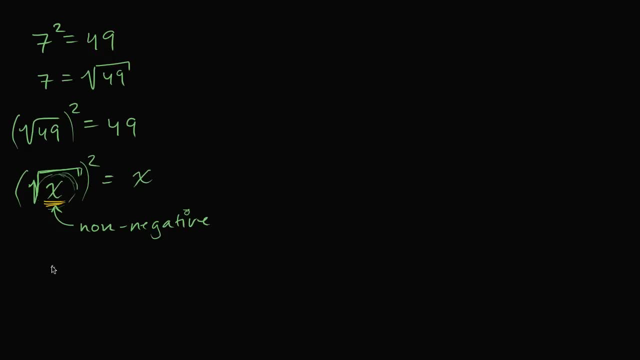 we need to put a non-negative number in here. But anyway, the focus of this video is not on the square root. it's really just to review things so we can start thinking about the cube root And, as you can imagine, where does the whole notion? 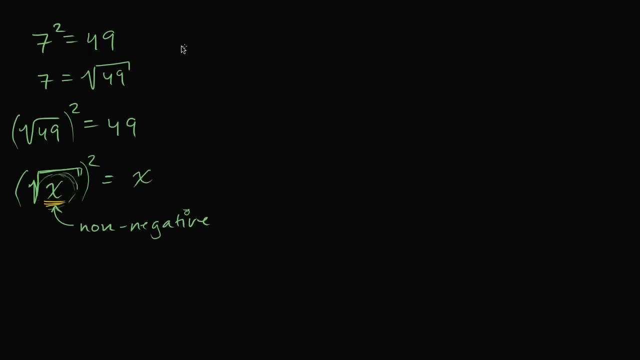 of taking a square of something or a square root come from? Well, it comes from the notion of finding the area of a square. If I have a square like this and if this side is seven, well, if it's a square. 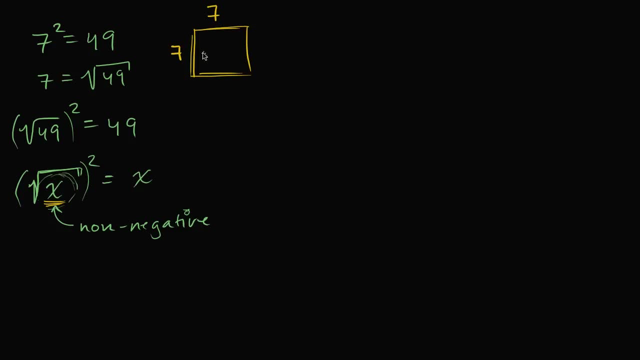 all the sides are going to be seven, And if I wanted to find the area of this, it would be seven times seven or seven squared. That would be the area of this. Or if I were to say: well, what is? 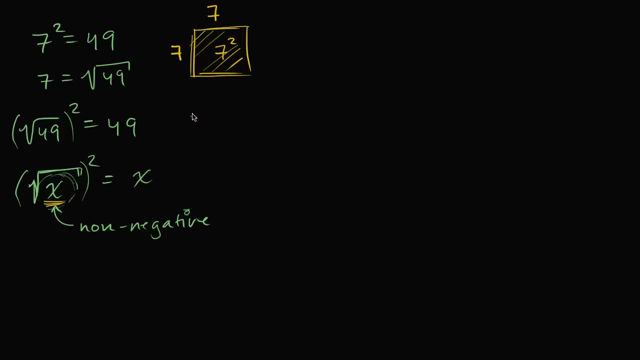 if I have a square, if I have- and that doesn't look like a perfect square, but you get the idea- all the sides are the same length. If I have a square with area x, if the area here is x, what are the lengths of the sides going to be? 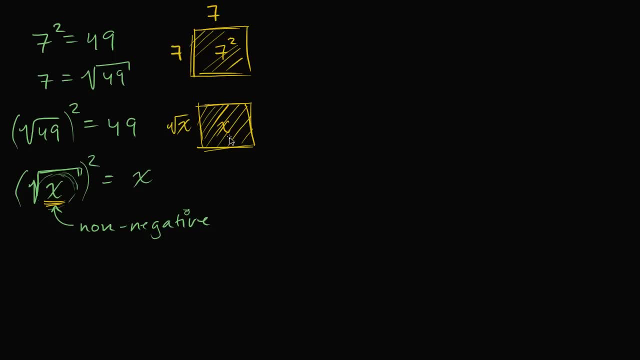 Well, it's going to be square root of x. All of the sides are going to be square root of x, So it's going to be square root of x by square root of x, and this side's going to be square root of x as well. 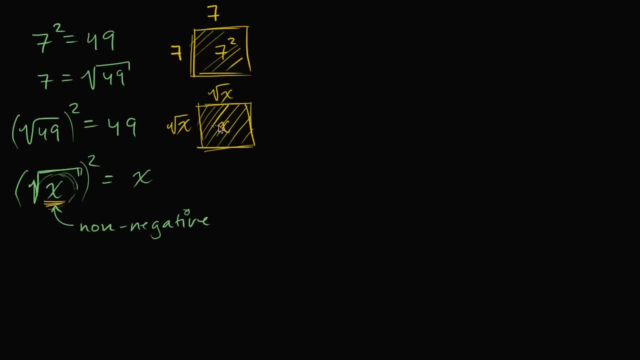 and that's going to be square root of x as well. So that's where the term square root comes from, where the square comes from. Now, what do you think? cube root? Well, same idea. If I have a cube, if I have a cube. 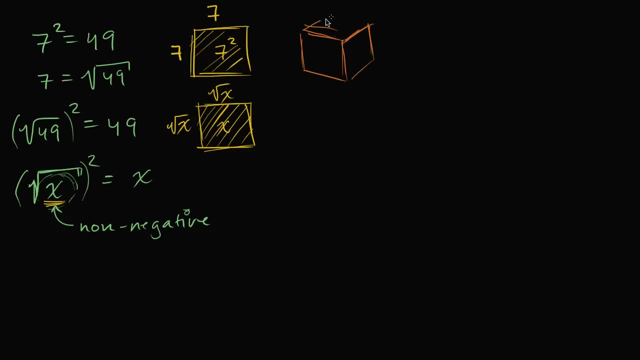 let me do my best attempt at drawing a cube really fast. If I have a cube and a cube, all of its dimensions have the same length. so this is a two by two by two cube. what's the volume over here? Well, the volume is going to be two times. two times two. 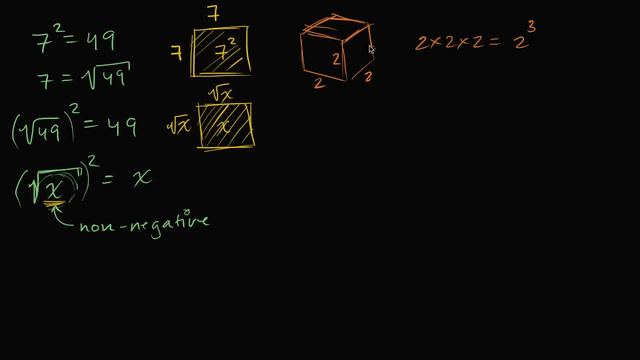 which is two to the third power, or two cubed. This is two cubed. That's why they use the word cubed, because this would be the volume of a cube where each of its sides have length two, and this, of course, is going to be equal to eight. 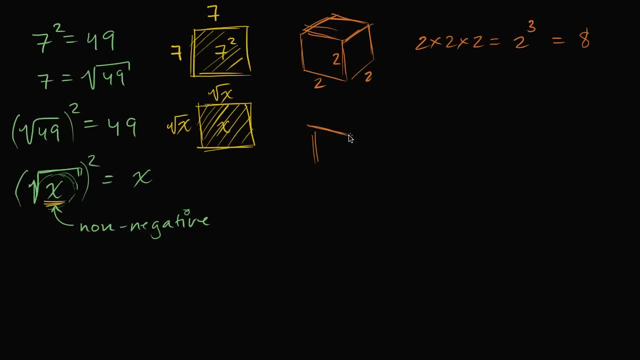 But what if we went the other way around? What if we started with the cube? or what if we started with its volume? What if we started with the cube's volume? and let's say the volume here is eight cubic units, so volume is equal to eight. 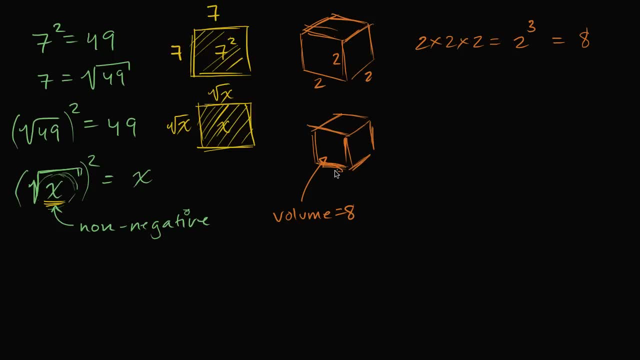 and we wanted to find the lengths of the sides. So we wanted to figure out what x is, because that's x, that's x and that's x. It's a cube, so all its dimensions have the same length. Well, there's two ways that we could express this. 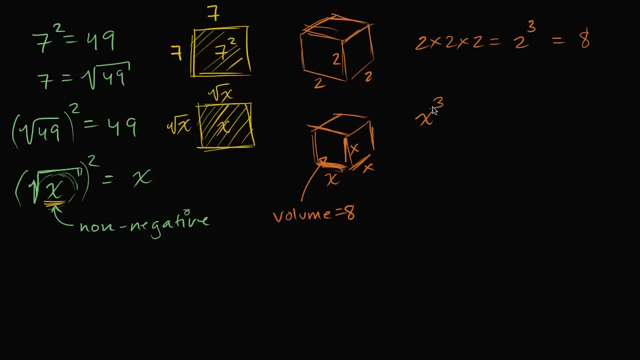 We could say that x times x times x, or x to the third power is equal to eight. or we could use the cube root symbol, which is a radical with a little three in the right place. or we could write that x is equal to. 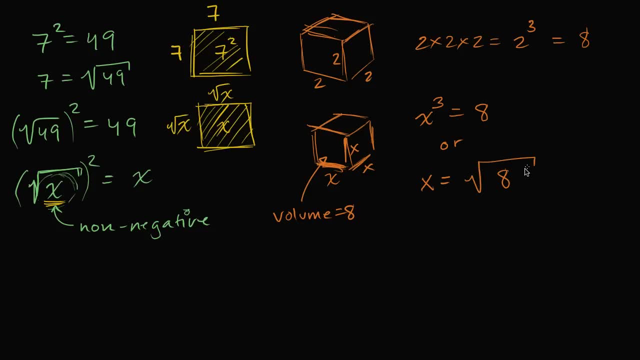 it's going to look very similar to the square root. this would be the square root of eight, but to make it clear that we're talking about the cube root of eight, we would write a little three over there, In theory for square root. 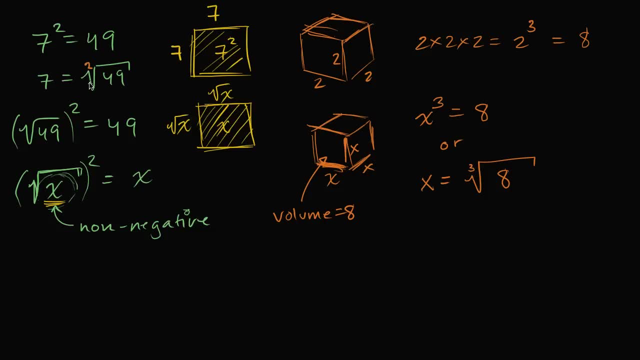 you could put a little two over here, but that'd be redundant. If there's no number here, people just assume that it's the square root. But if you're figuring out the cube root, or sometimes people say the third root, well then you have to say: 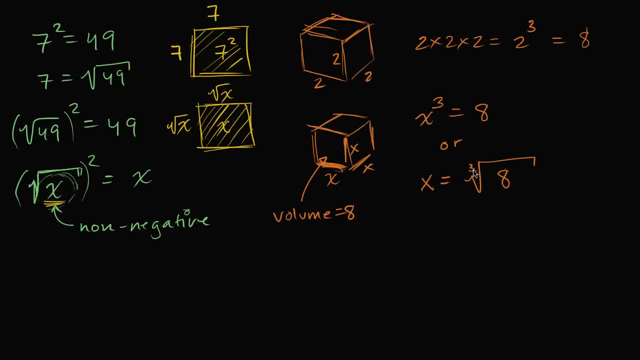 well, you have to put this little three right over here and this little notch in the radical symbol right over here, And so this is saying x is going to be some number that if I cube it I get eight. So with that out of the way, let's do some examples. 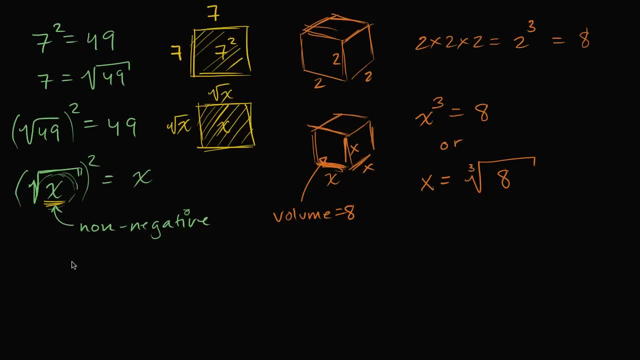 Let's say that I have, let's say that I want to calculate the cube root of 27.. What's that going to be? Well, if I say that this is going to be equal to x, this is equivalent to saying that x to the third. 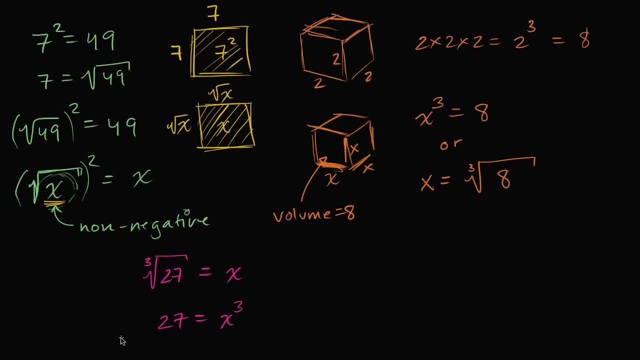 or that 27 is equal to x to the third power. So what is x going to be? Well, x times x times x is equal to 27.. Well, the number I can think of is three, So we would say that x. 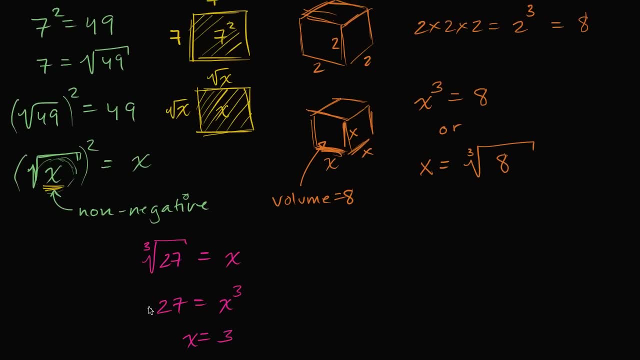 let me scroll down a little bit. x is equal to 27.. Three, Now let me ask you a question: Can we write? can we write something like: can we pick a new color? The cube root of? let me write: negative 64.. 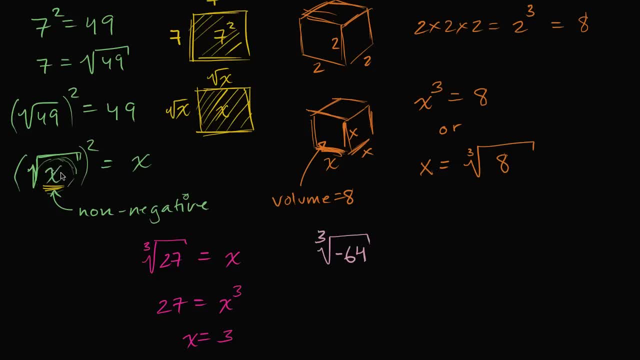 I already talked about that. if we're talking the square root, it's fairly typical that, hey, you put a negative number in there, at least until we learn about imaginary numbers, we don't know what to do with it. But can we do something with this? 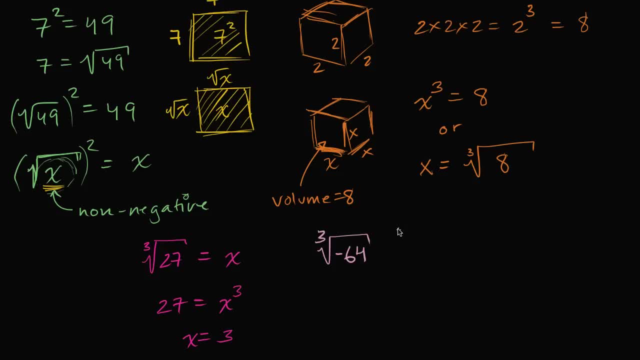 Well, if I multiply, if I cube something, can I get a negative number? Sure, If I take. so, if I say this is equal to x, this is the same thing as saying that negative 64 is equal to x. to the third power. 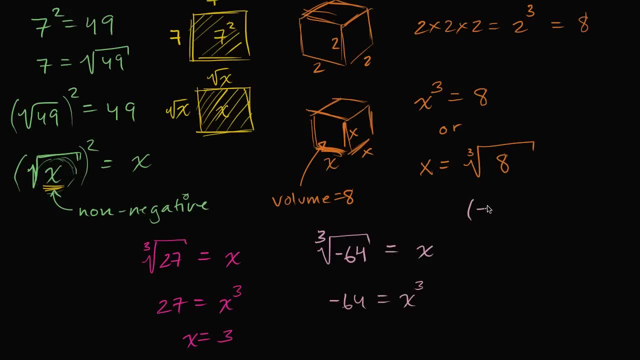 Well, what could x be? Well, what happens? if you take negative four times negative, four times negative, four Negative four times negative, four is positive 16, but then times negative four is negative 64, is equal to negative 64.. So what could x be here? 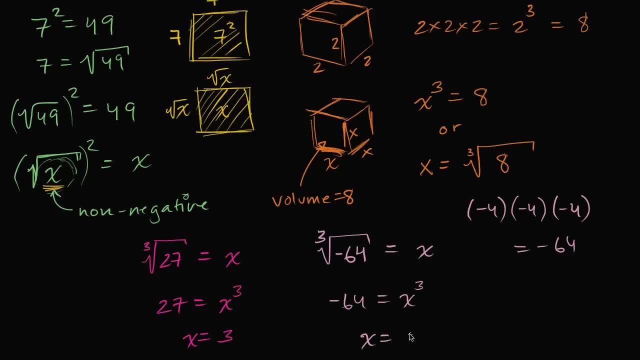 Well, x could be equal to negative four. x could be equal to negative four. So, based on the math that we know so far, you actually can take the cube root of a negative number. And just so you know, you don't have to stop there. 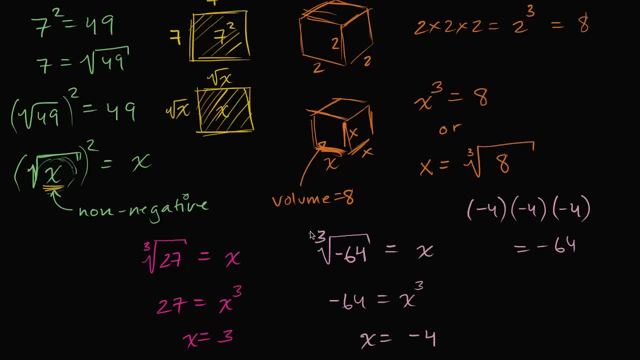 You could take a fourth root and in this case you would have a four here, a fifth root, a sixth root, a seventh root of numbers- And we'll talk about that in well later in your mathematical career. But most of what you're gonna see, 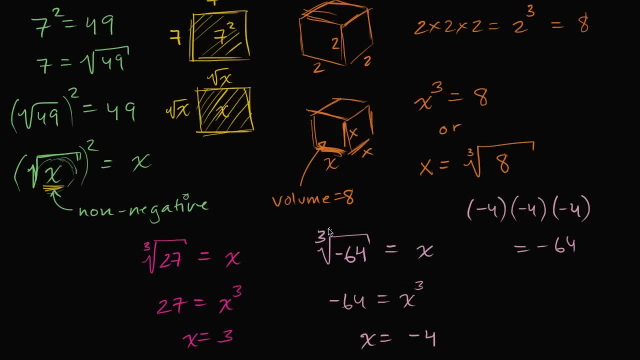 is actually going to be square root and every now and then you're going to see a cube root. Now you might be saying: well, hey look, you just knew that three to the third power is 27.. You took the cube root, you get x. 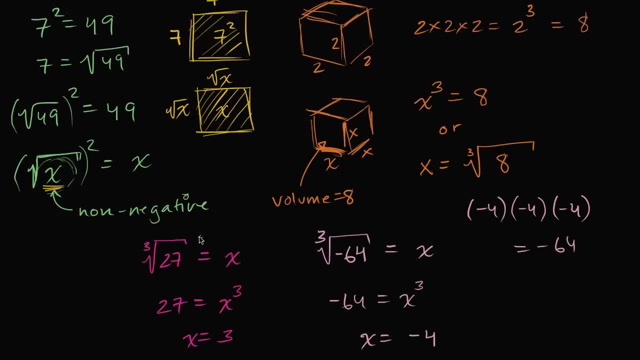 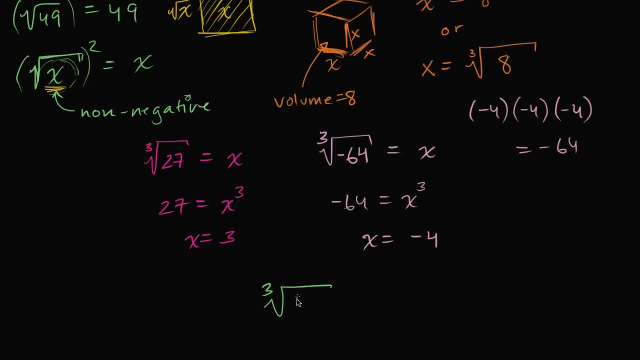 Is there any simple way to do this? And, like you know, if I give you an arbitrary number, if I were to just say, I don't know if I were to say cube root of 125.. And the simple answer is well. 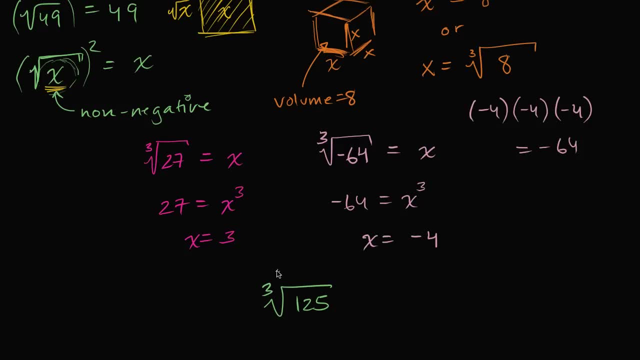 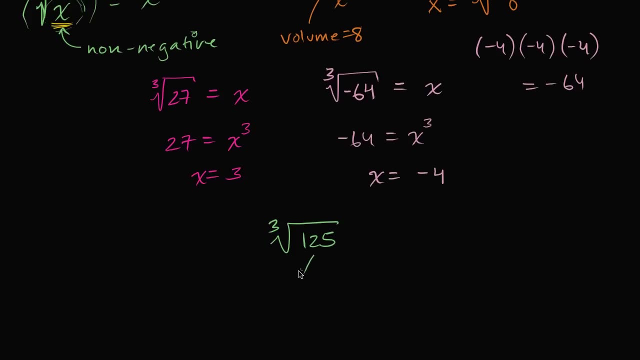 the easiest way to actually figure this out is actually just to do a factorization, in particular a prime factorization, of this thing right over here, and then you would figure it out. So you would say: okay, well, 125 is five times 25,.